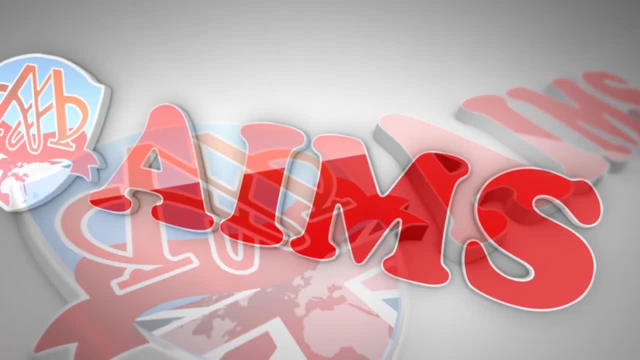 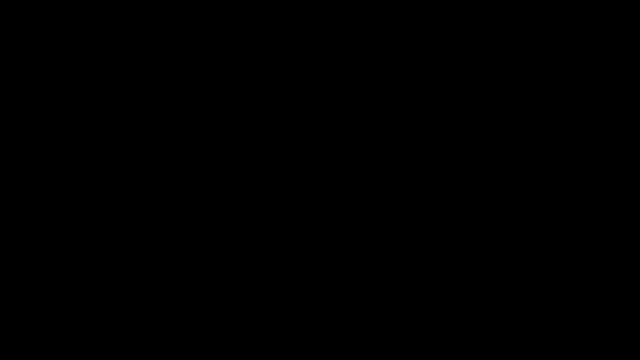 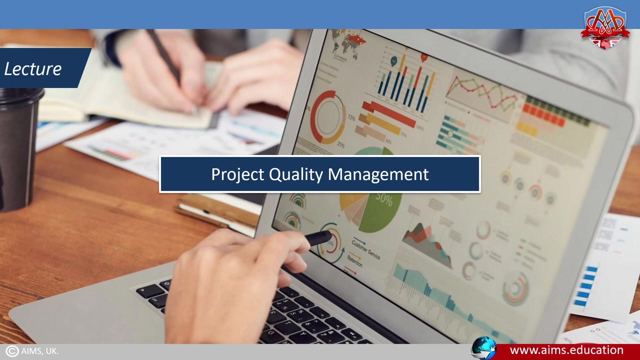 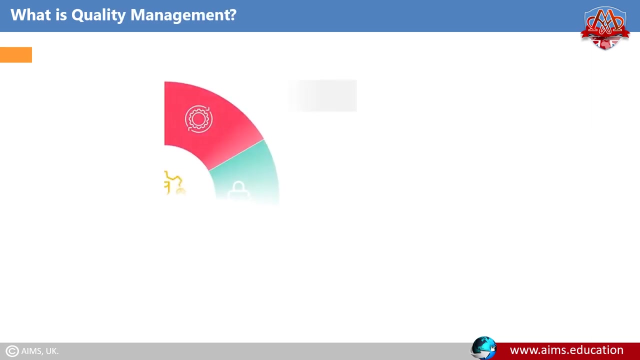 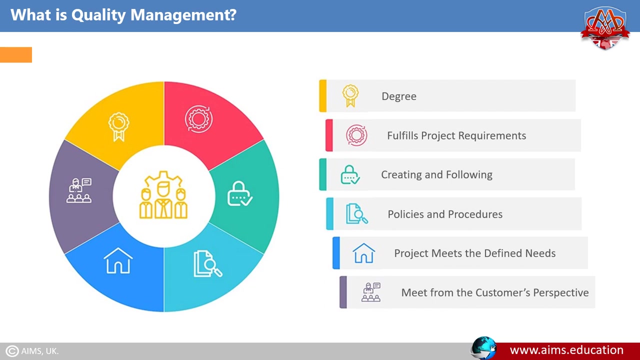 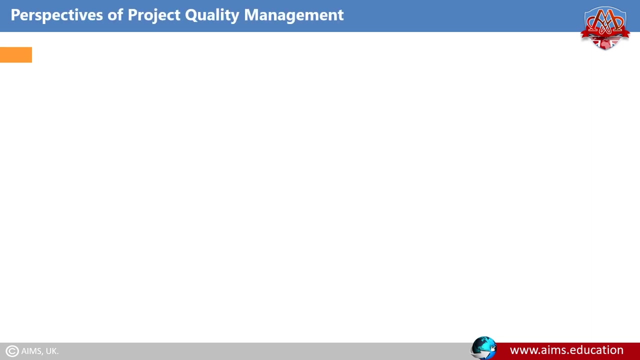 What is Quality Management? Quality is the degree to which the project fulfils requirements. Quality management includes creating and following policies and procedures in order to ensure that a project meets the defined needs it was intended to meet from the customer's perspective. Here are some perspectives of project quality management. 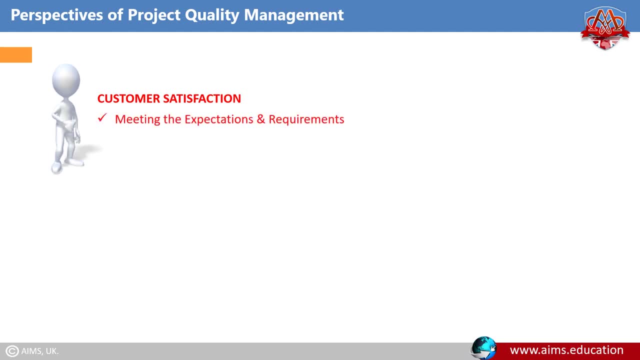 Customer Satisfaction. Quality is all about meeting the expectations and requirements of the customer and stakeholders and creating a product that fulfils those needs and is fit for its intended use. Prevention Quality is achieved by planning, designing and building it into a product or process from the inception. 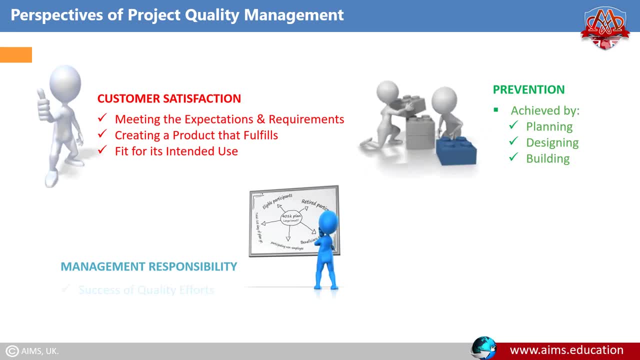 Management Responsibility. The project team must ensure the success of quality efforts and the organizational management must provide the financial resources needed for quality efforts to succeed. Continuous Improvement, Quality and process improvement relies on the ongoing plan. do check and act cycle. Quality Management, Understanding Quality and Grade. 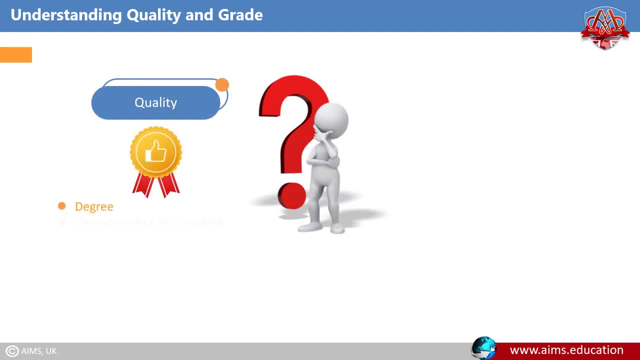 Quality. Quality is the degree to which the characteristics of a product meet the demands or expectations of the project. In other words, quality is conformance to the requirements, including the product and customer's requirements. Grade Grade is a category or rank assigned to products or services having the same functional use. 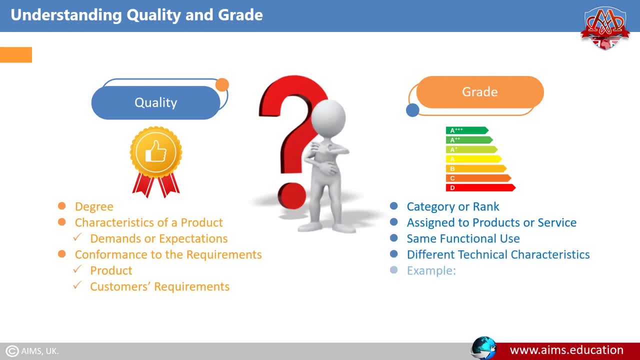 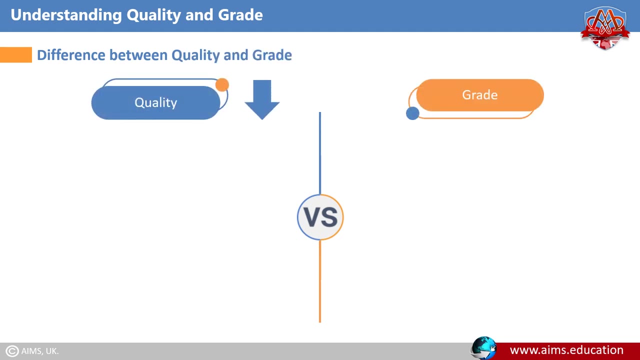 but different technical characteristics. For example, there are different grades of paint, different grades of metal and even different grades of travel Quality and Grade. Low quality does not equal to low grade. Low quality is usually not acceptable, but on the other hand, low grade is never a problem and it is acceptable. 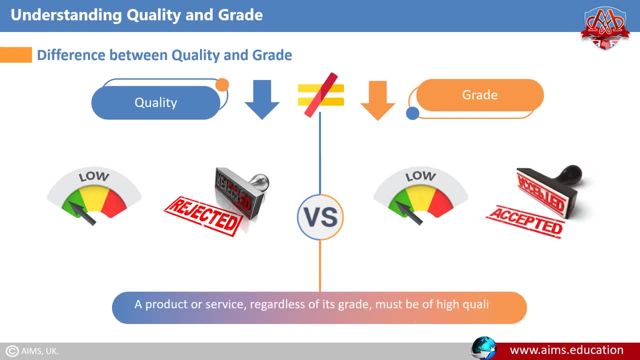 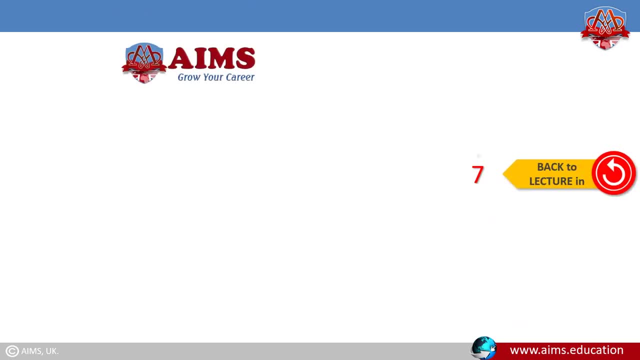 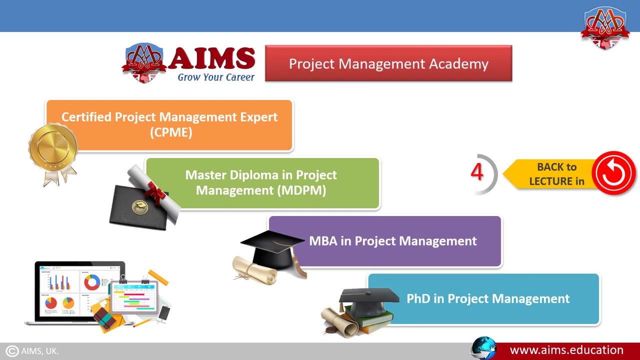 Product or Service. Product or Service grade must be of high quality. AIMS is a globally recognized and an accredited institution. We offer certifications, diploma, MBA and PhD programs in project management through an online and self-paced learning system. For registration and details, please visit wwwaimseducation. 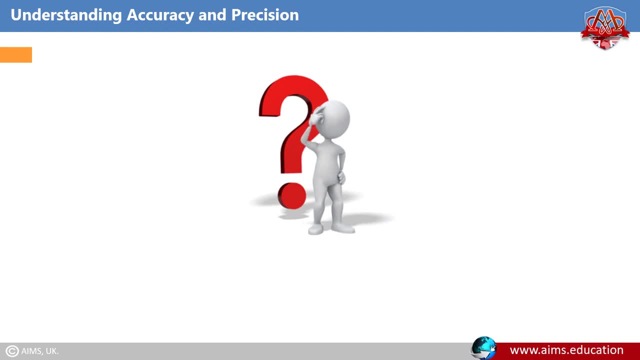 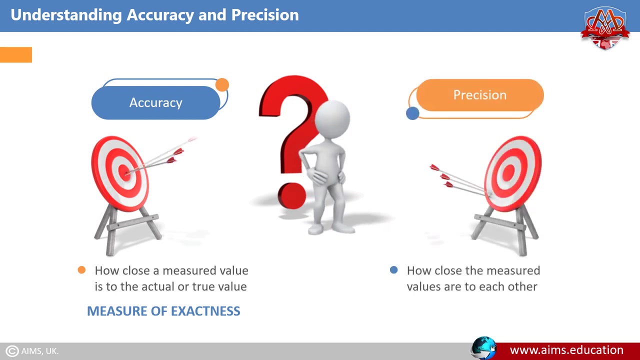 Understanding Accuracy and Precision. Accuracy: It represents how close a measured value is to the actual or true value. Accuracy is the measure of exactness. And Precision: It represents how close the measured values are to each other. Precision is an assessment of correctness. 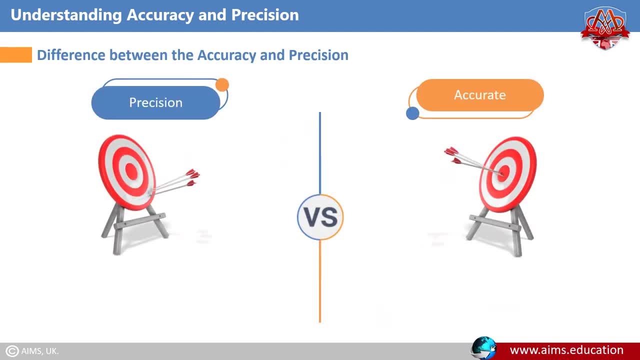 Difference between Accuracy and Precision. Measured values may or may not be near the actual or true value, but they are the same. But if the scatter is lesser, the measurements are said to have a high precision. When measurements are close to the target value, they are accurate. 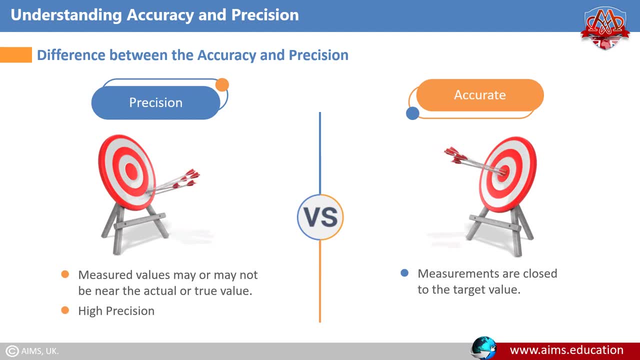 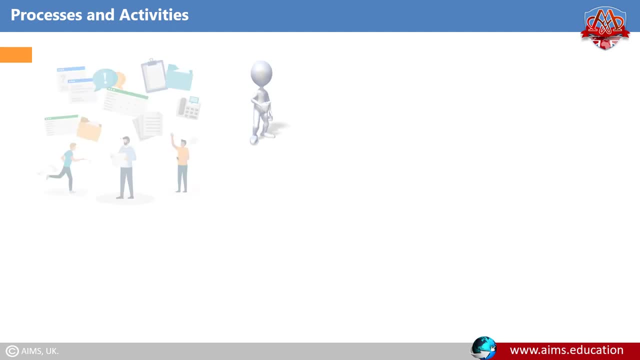 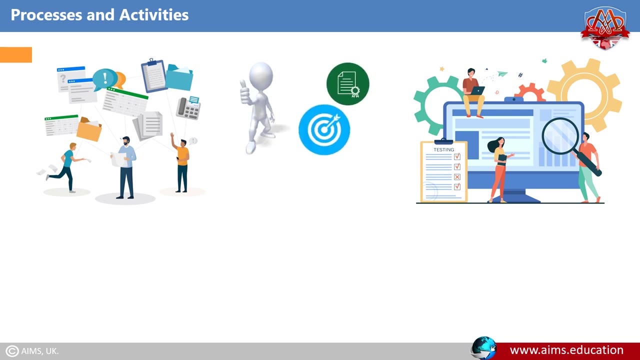 Scatter does not have any significant role here. Processes and Activities In order to satisfy the project needs. the processes and activities of project quality management determine quality policies, objectives and responsibilities. There are three core project needs: Project Quality Management, Processes, Plan Quality Management. 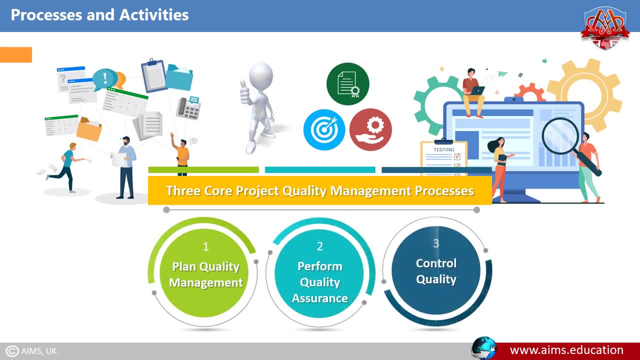 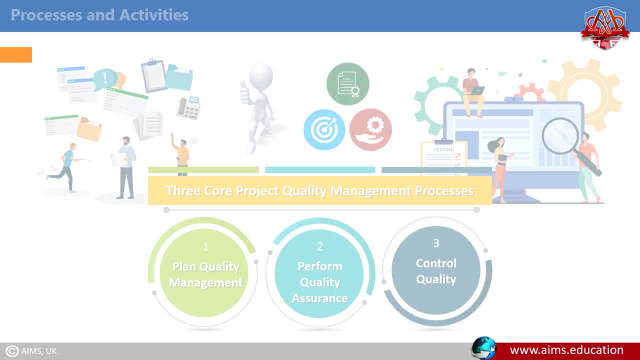 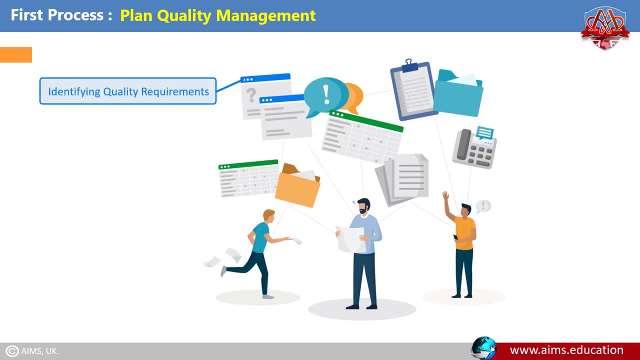 Perform Quality Assurance, Control, Quality. We will now understand each of these processes in more detail. First Process Plan: Quality Management. It is the process of identifying quality requirements and or standards for the project and its deliverables and documenting how the project will demonstrate compliance with relevant quality requirements. 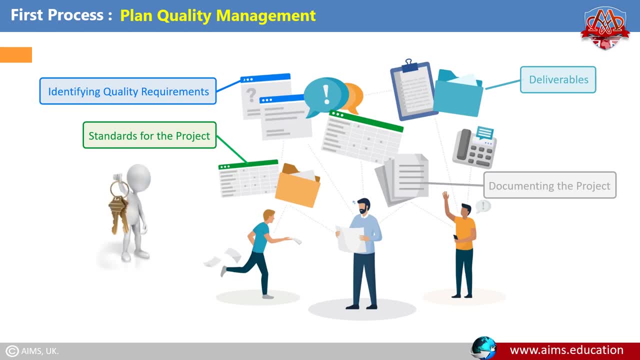 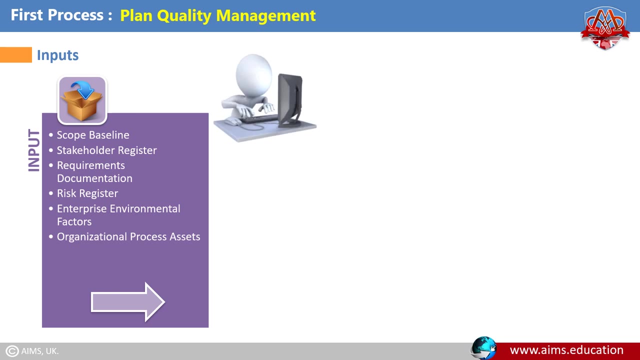 Key Benefit. This process provides guidance and direction on how quality will be managed and validated throughout the project. Inputs for Plan Quality Management. The inputs to create the plan quality management are: Scope Baseline, Stakeholder Register, Requirements, Documentation, Risk Register, Enterprise, Environmental Factors and Organizational Processes. 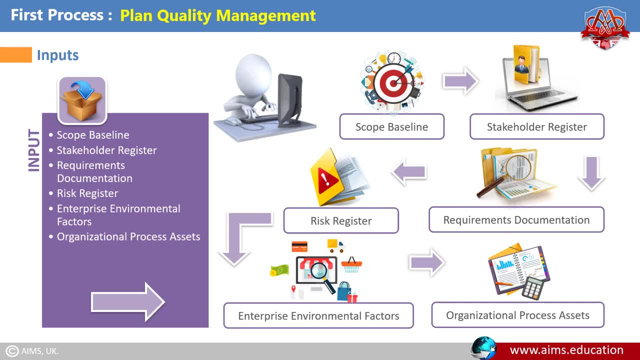 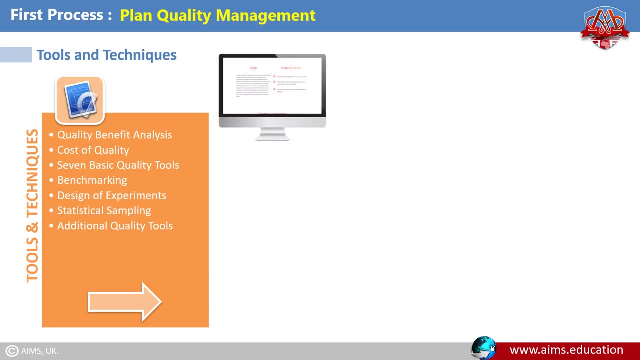 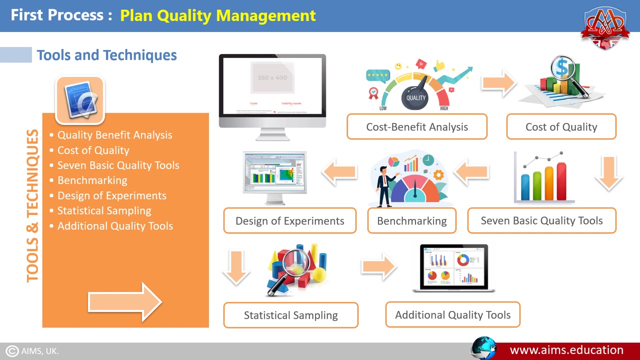 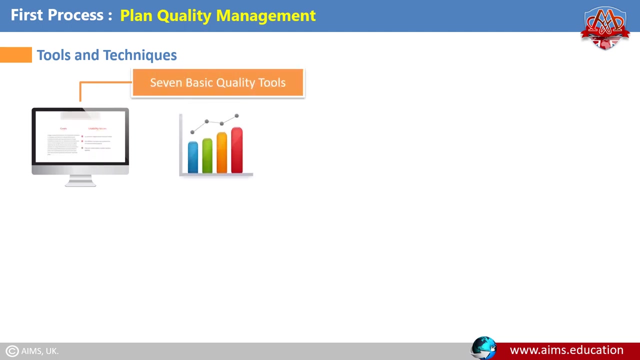 Inputs for Plan Quality Management Tools and techniques for plan quality management. Tools and techniques to create the plan quality management are: Cost benefit analysis, Cost of quality- Seven basic quality tools, Benchmarking, The design of experiments, Statistical sampling And additional quality tools. The plan quality management process. The Seven Basic Quality Tools. 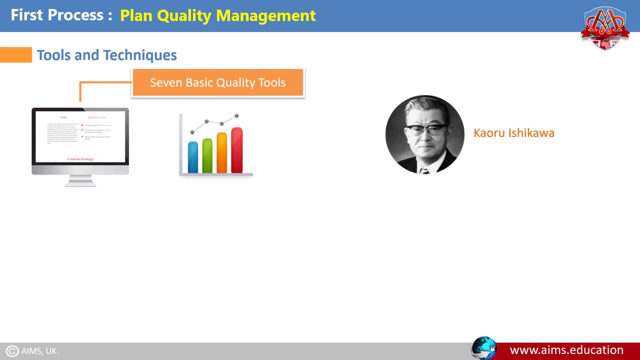 Kaoru Ishikawa was a Japanese organizational theorist and well known for his quality management innovations. He developed seven basic visual tools of quality so that the average person could analyze and interpret data. These seven tools are a cause and effect diagram, flow charts. 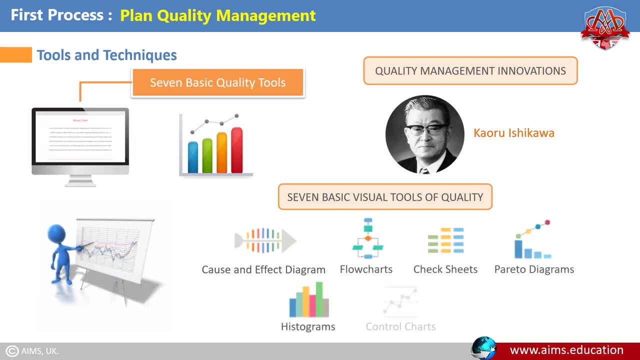 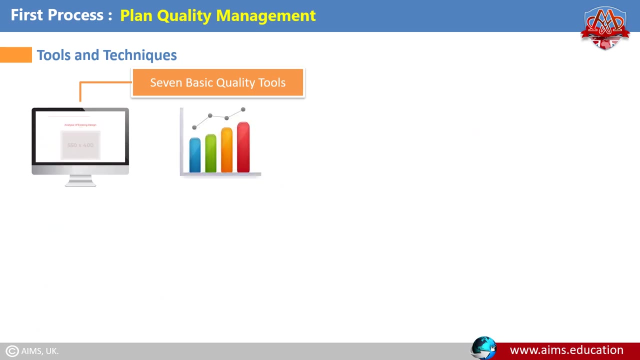 check sheets, Pareto diagrams, histograms, control charts and scatter diagrams. These tools are used worldwide by companies, managers of all levels and employees. The First Basic Quality Tool: The Cause and Effect Diagram. The Cause and Effect Diagram is also called the Fishbone Diagram. 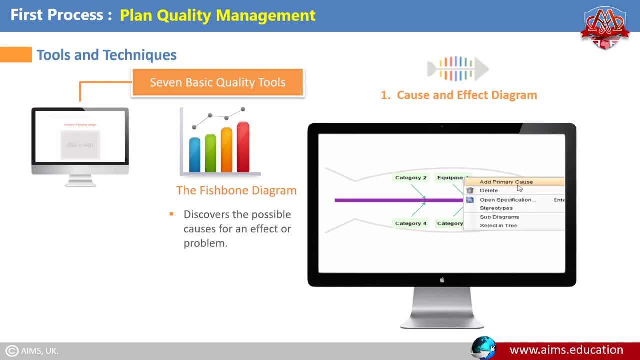 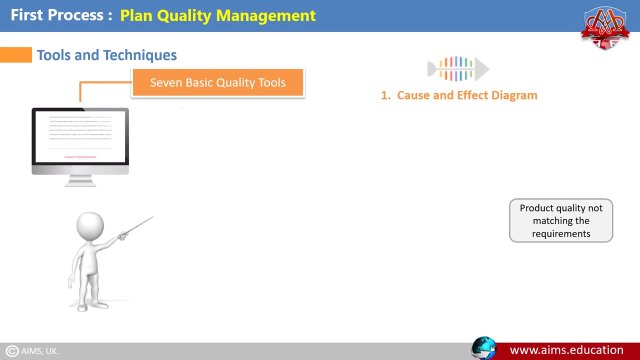 This tool discovers the possible causes for an effect or problem. This diagram acts as a first step in problem solving by creating a list of possible causes. Let's see how the Fishbone Diagram works. First, clearly identify and define the problem or effect for which the causes must be identified. 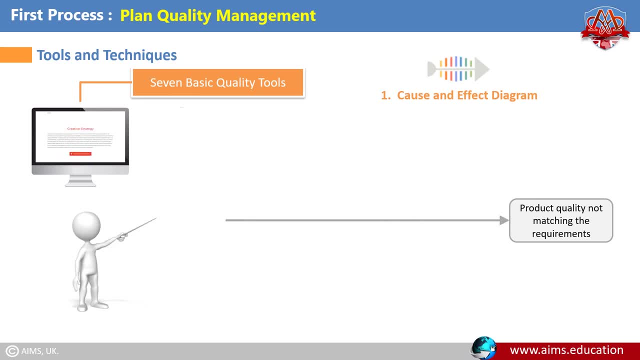 Place the problem or effect at the right or the head of the diagram. Then identify all the broad areas of the problem. Then write the possible causes in each of the broad areas. Each cause that has been identified should now look for more causes. Now view the. 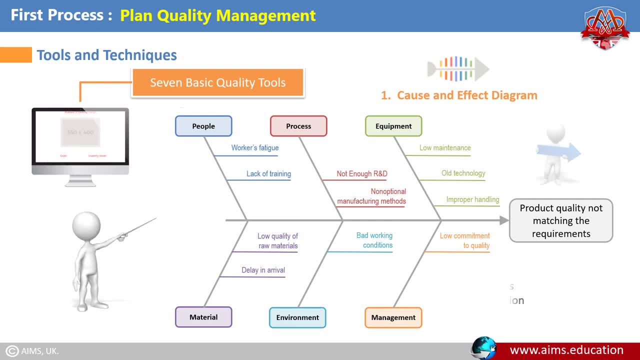 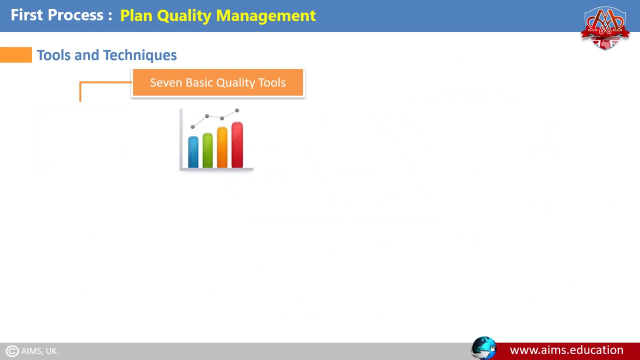 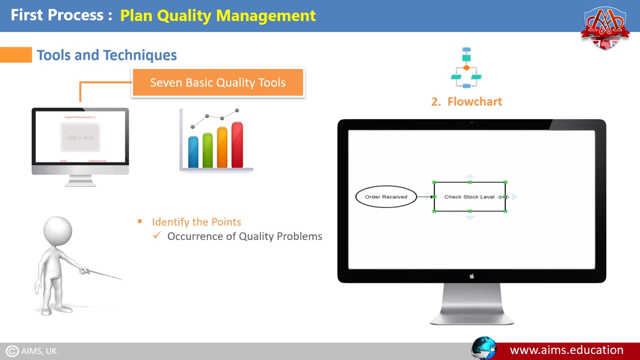 diagram and evaluate the main causes And finally set goals and take action on the main causes. First, Basic Quality Tool. Second, basic quality tool: Flowchart. It is a graphical representation of a process and it shows the relationships among process steps. It can help a project to identify the points where quality problems might occur. 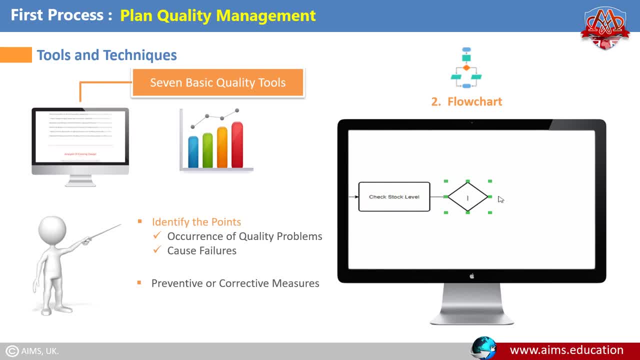 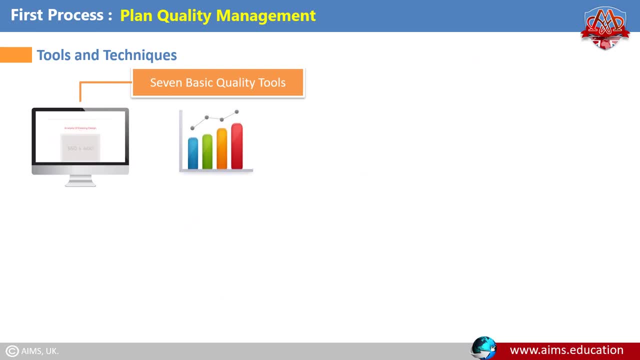 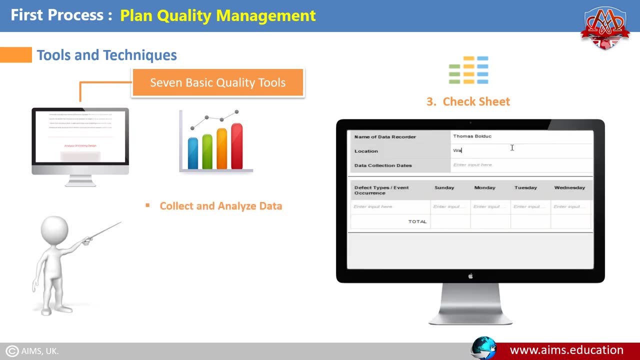 and may cause failures. Preventive or corrective measures can be taken to avoid problems. Third Basic Quality Tool: The Third Basic Quality Tool, Checksheet. A checksheet is a structured form that's prepared to collect and analyze data, which leads us to organize facts about a potential quality problem. 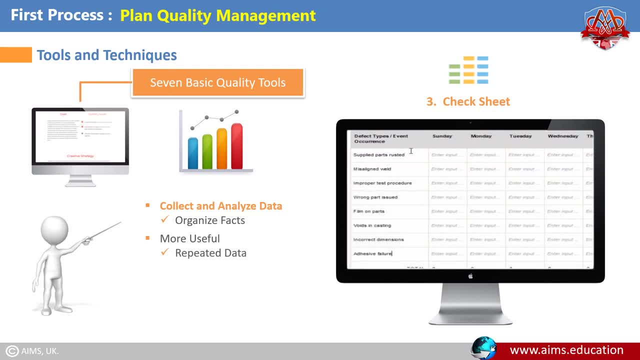 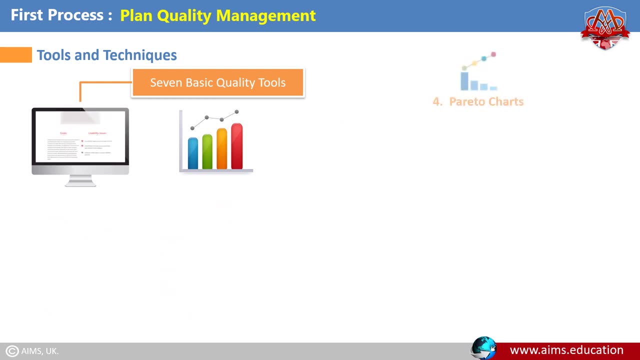 It's more useful when repeated data is collected from the same person or effect. For example, a checksheet is used to collect data about the frequencies or consequences of defects. The fourth basic quality tool: Pareto charts. These are used to identify and prioritize problems to be solved. 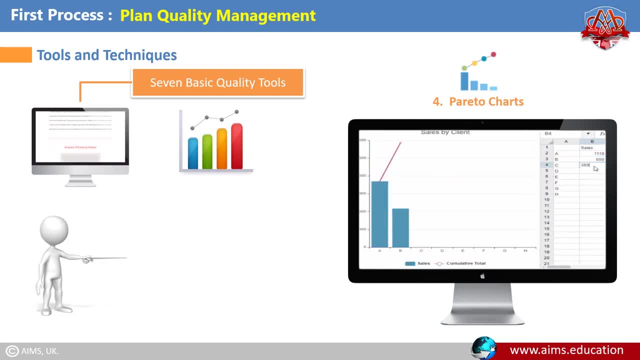 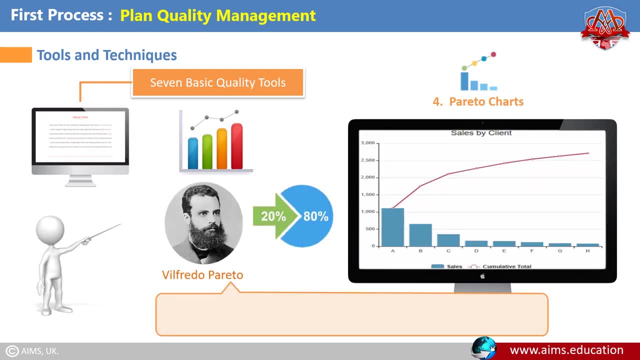 They are actually histograms, aided by the 80-20 rule introduced by Vilfrido Pareto. The 80-20 rule, as it applies to quality, says that 80% of the problems or outputs come from 20% of the causes or inputs. 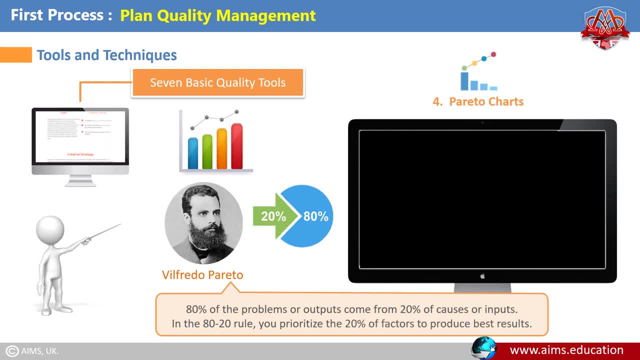 In the 80-20 rule, you prioritize the 20% of the factors to produce the best results. Pareto charts are displayed as histograms. They are histograms that rank order the most important factors by their frequency over time. The fifth basic quality tool: Histograms. 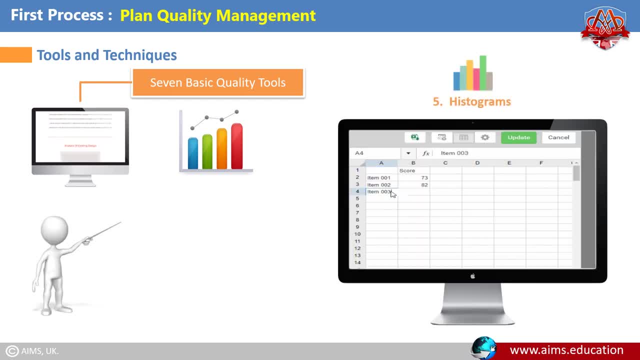 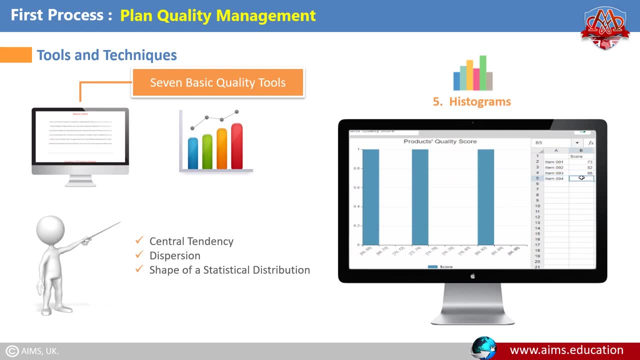 They are a special form of bar chart and are used to describe the central tendency, dispersion and shape of a statistical distribution. Unlike the control chart, the histogram does not consider the influence of time on the variation that exists within a distribution. The sixth basic quality tool: Control Chart. 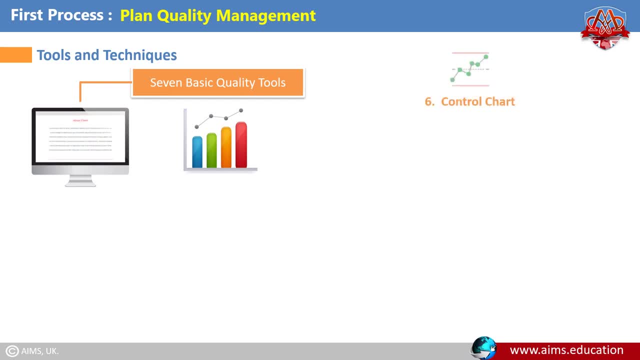 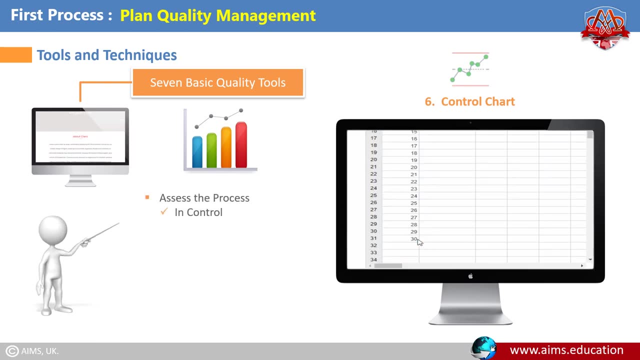 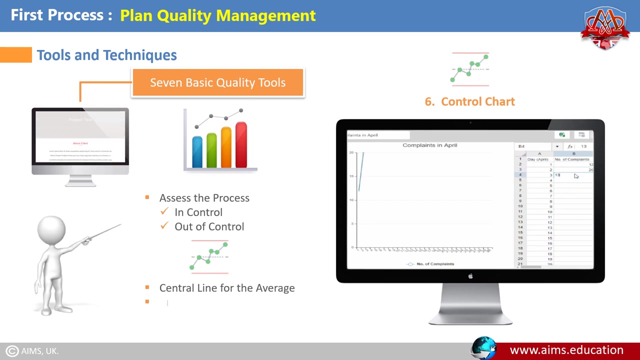 The sixth basic quality tool, Control chart. A graphical display of the results over time of a process is used to assess whether the process is in control or it is out of control. A control chart always has the following: A central line for the average, an upper line for the upper control limit and a lower line for the lower control limit. 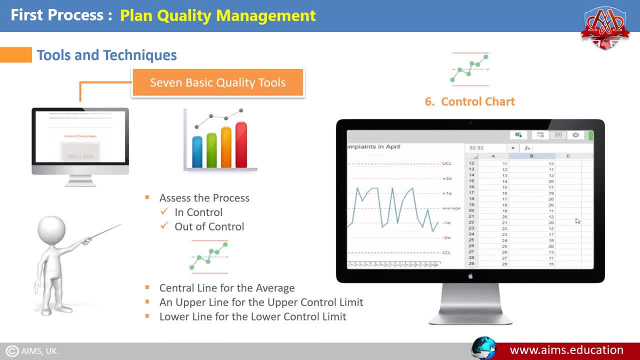 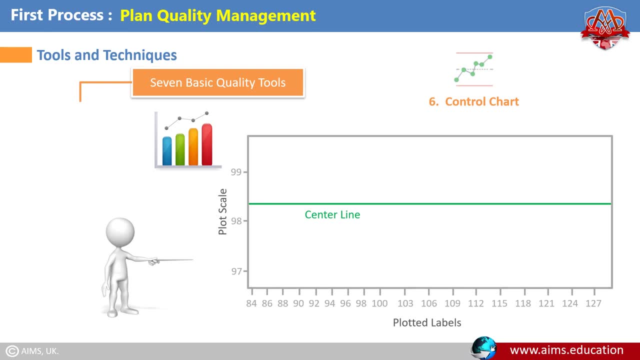 These lines are determined from the historical data. In this chart, you may observe that the central line is surrounded by two more lines, and they are known as the upper specification limit and the lower specification limit. The upper and lower specification limits are provided in the contract and one cannot cross. 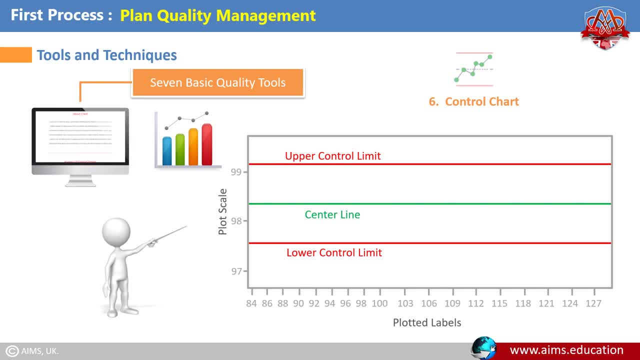 them. The upper and lower control limits are determined by the project manager. By comparing current data to these limits, you can draw conclusions about whether the process variation is consistent or is unpredictable. If 99.73% of all the points fall between the upper and lower control limits, the project 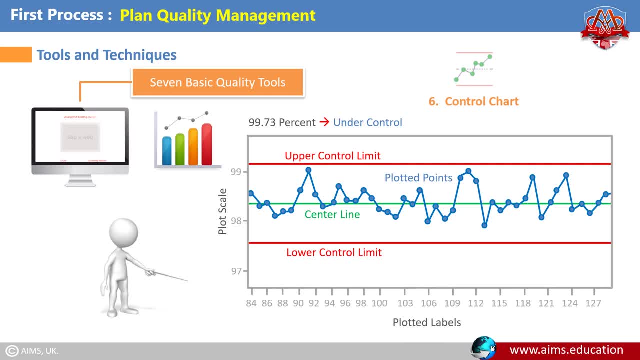 is considered as under control The rule of seven. If seven or more consecutive data points fall on one side of the mean, then an investigation must be initiated to find out the reason for it, even if these points fall within the control limits. This is known as the rule of seven. 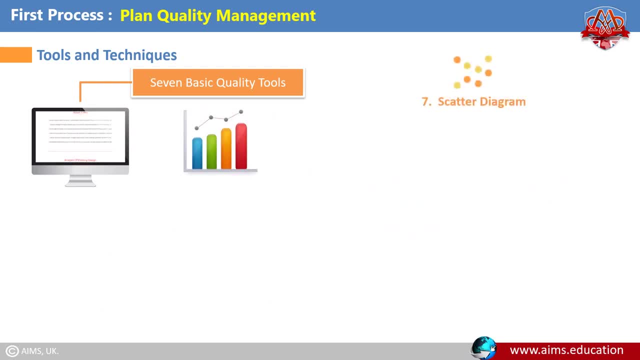 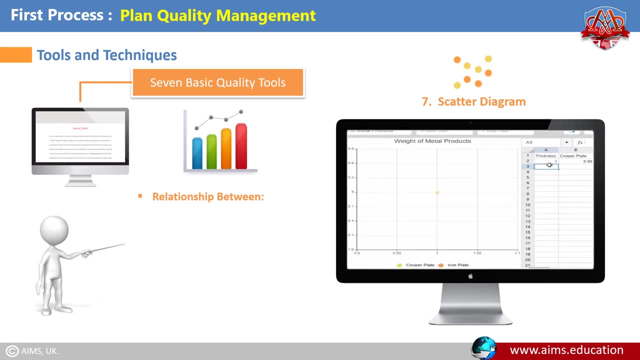 And the seventh basic quality tool, a scatter diagram. It is a graph that shows the relationship between two variables. Scatter diagrams can show a relationship between any element of a process, environment or activity on one axis and a quality defect on the other axis. 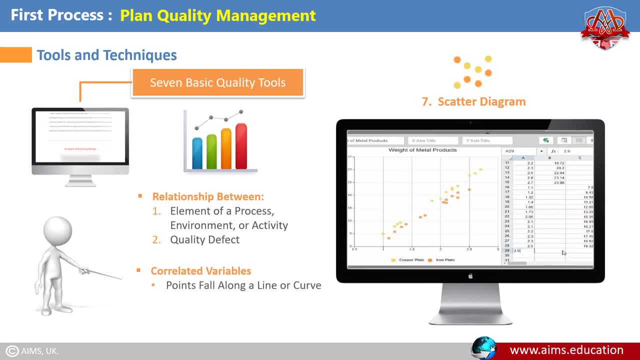 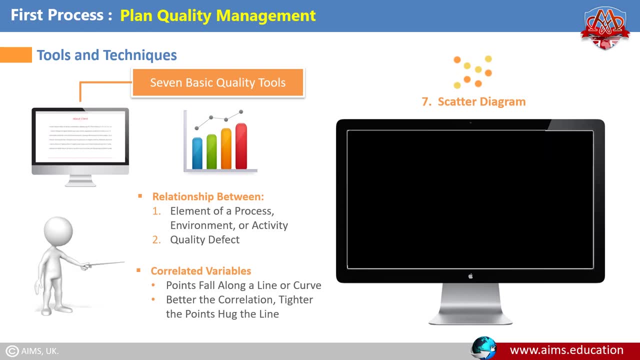 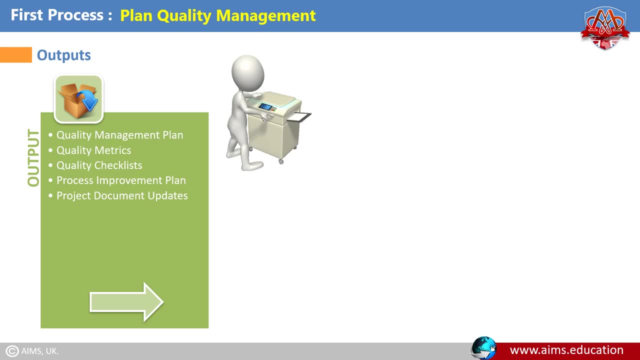 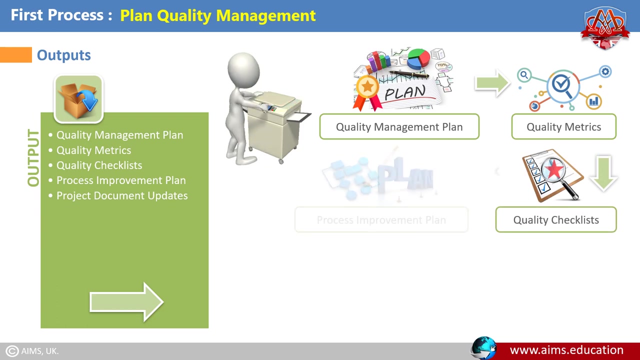 If the variables are correlated, the points will fall along a line. The better the correlation, the tighter the points will hug the line. Outputs of Plan Quality Management. Outputs to create the Plan Quality Management are: Quality Management Plan, Quality Metrics, Quality Checklists, Process Improvement Plan. 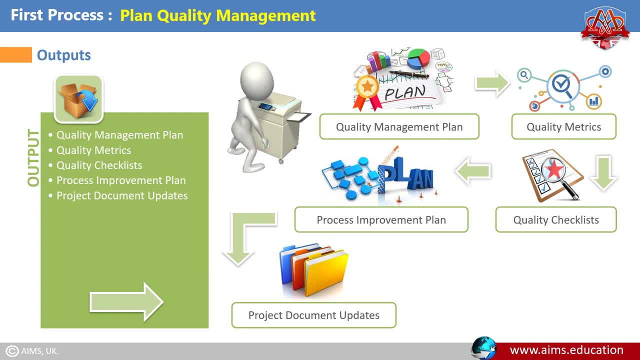 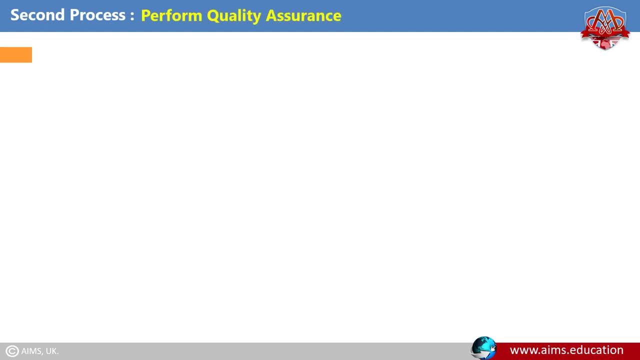 and Project Document Updates. Outputs of Plan Quality Management. Outputs to create the Plan Quality Management. Second process: Perform Quality Assurance. Quality assurance is sandwiched between Plan Quality Management and Control Quality. This is how it is done. First, you plan the quality processes, policies, techniques, methods and metrics. 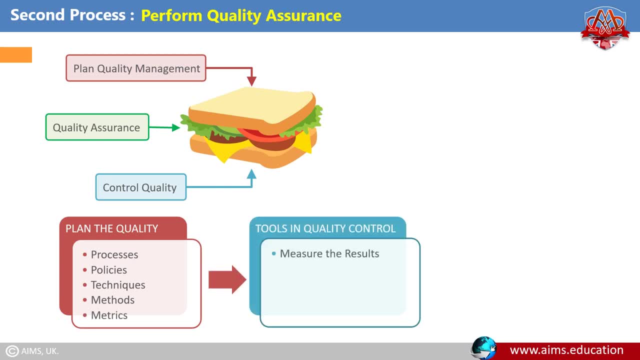 Then using the tools. in quality control, you measure the results by using the identified tools, techniques and methods to see whether they comply with the identified metrics. Finally, in Quality Assurance, you identify whether the process is working and if there are ways to improve it. 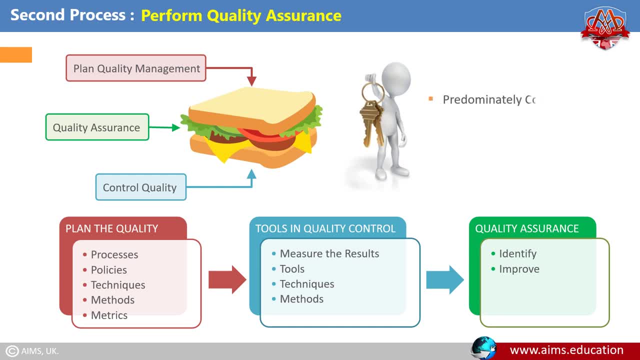 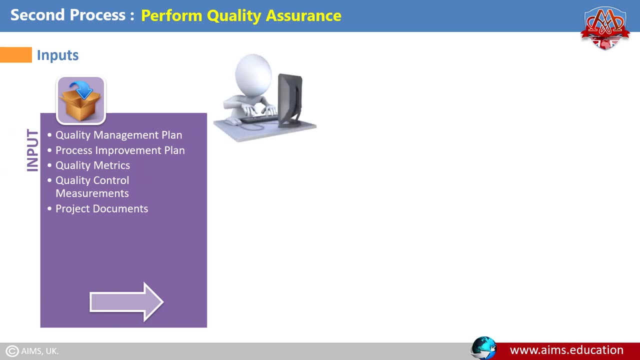 Key Benefit. Quality Assurance is predominantly concerned with improving processes and it leads to improved results. Inputs for Perform Quality Assurance. Inputs for the Perform Quality Assurance process come from Plan Quality Management and the Control Quality processes. They are: Quality Management, Plan Process, Improvement Plan Quality Metrics, Quality. 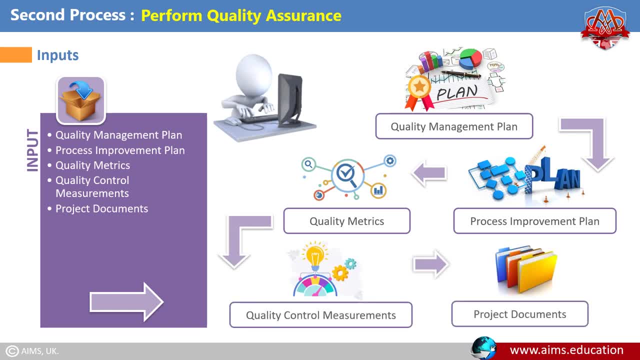 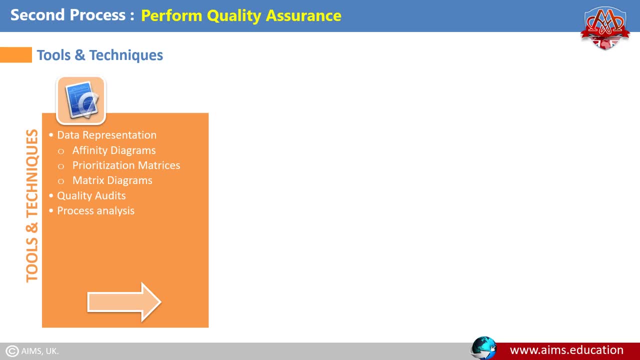 Control Measurements and Project Documents. Tools and Techniques for Perform Quality Assurance. Perform Quality Assurance is concerned with Process Improvement – the same tools and techniques of Plan Quality Management and Control Quality Procedures. control quality can help in this perform quality assurance process. the difference is that they're 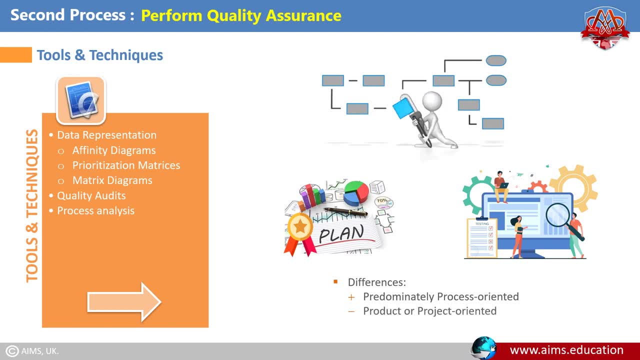 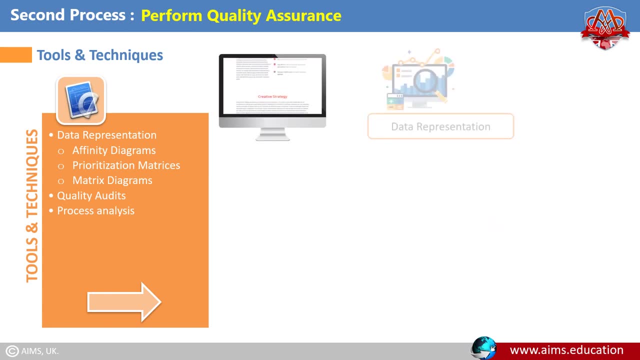 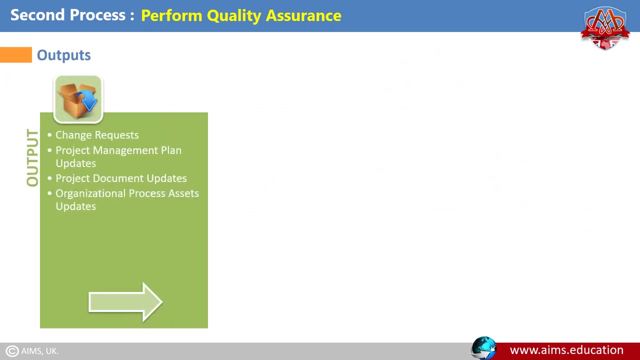 predominantly process oriented rather than product or project oriented. in addition to the previously discussed tools and techniques, the following quality management tools are used: affinity diagrams, prioritization matrices, Matrix diagrams, quality audits and process analysis. outputs of perform quality assurance, the intended outcome of quality audit and process improvement. 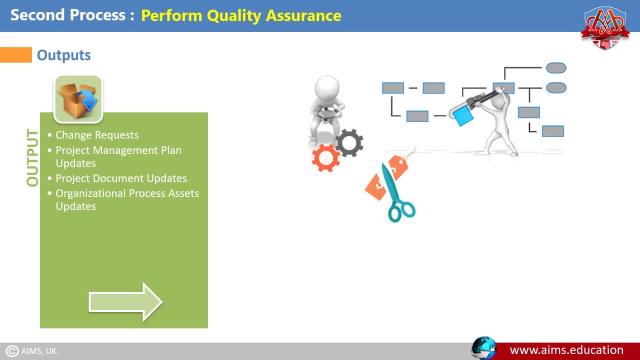 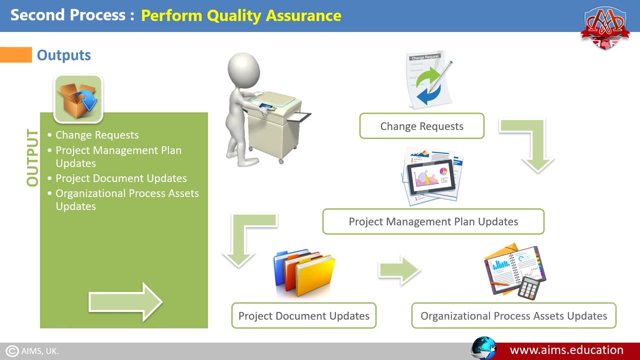 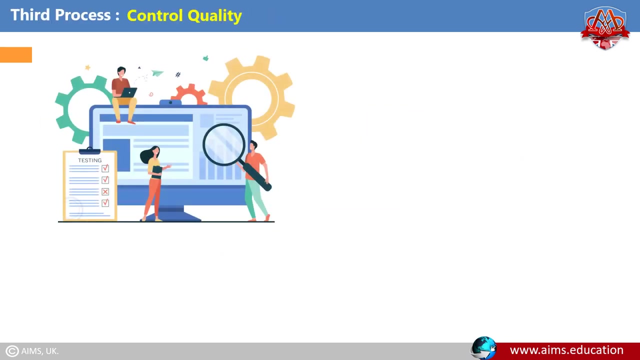 activities is to reduce the cost of quality and or to increase customer satisfaction. the outputs of perform quality assurance are change requests, project management plan updates, project document updates and organizational process asset updates. third process, control quality. it is a process of inspecting and verifying the product and services. 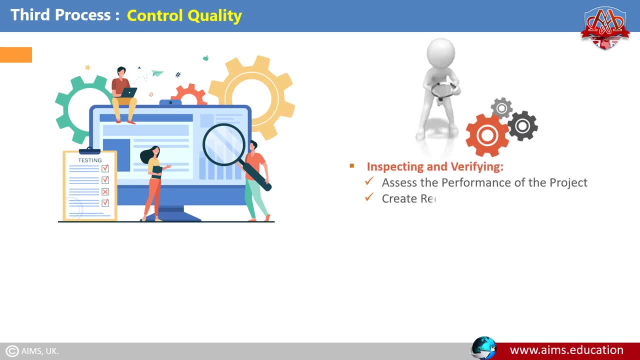 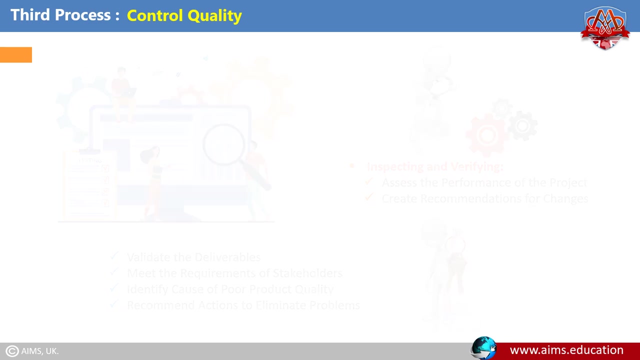 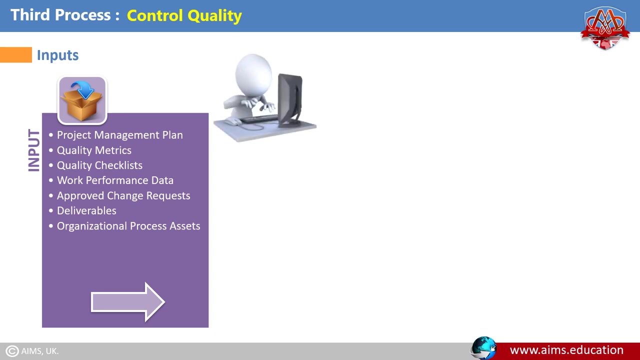 in order to assess the performance of the project and create recommendations for changes. here are the benefits of control quality: validate the deliverables, meet the requirements as specified by the stakeholders, identify causes of poor product quality and recommend actions to eliminate problems related to quality. inputs for perform quality control process. here are the inputs of perform quality process.